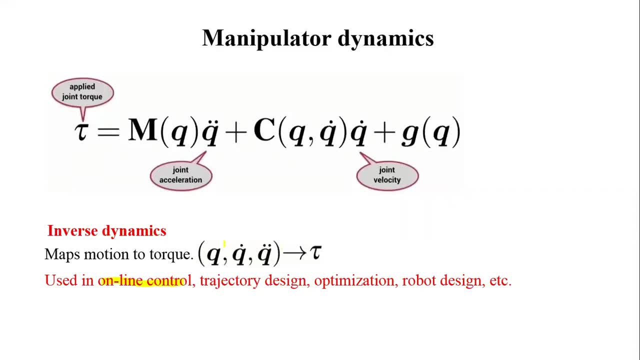 control. these motion variables are taken as feedback signals and the controller. they are used to calculate the torque required torque, after need to be need to be applied in trajectory design. these motion variables q, q, dot and two double dot are planned for generating a required torque. this relationship also helps to optimize the manipulator parameters. in order to obtain 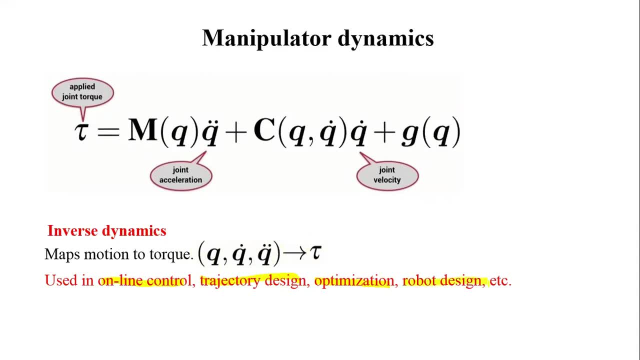 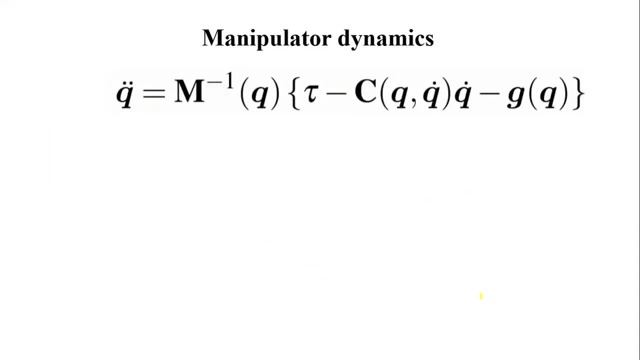 best torque. it is also used in robot design, and there are so many other applications as well. there is another form of manipulator dynamics and this: this form of manipulator dynamics is used to calculate motion variables from the applied torque. so forward dynamics must start to motion. it is used to simulate robot motion. 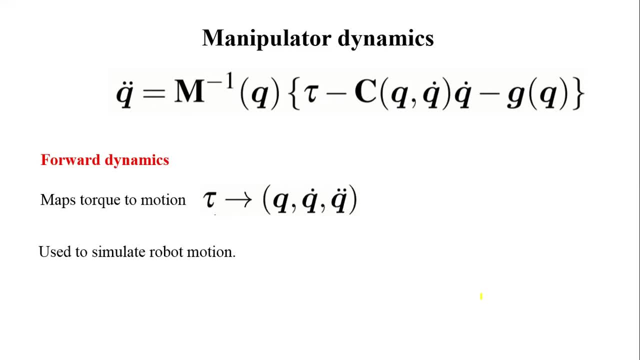 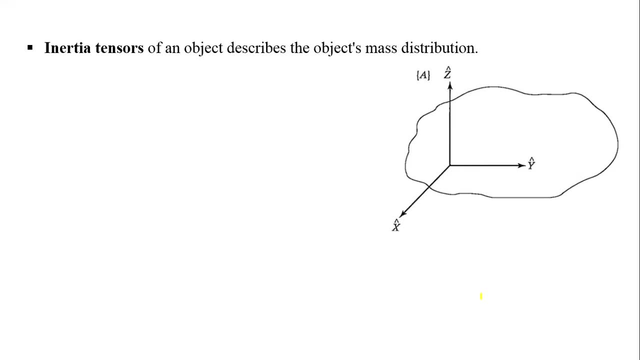 simulate, or simulation means mimicking natural behavior of any system, the mass, the manipulator, dynamics required. some system properties like mass of the manipulator, then it may require, require damping of the manipulator and also stiffness. these system properties like mass, stiffness and damping are written in the form of matrices. 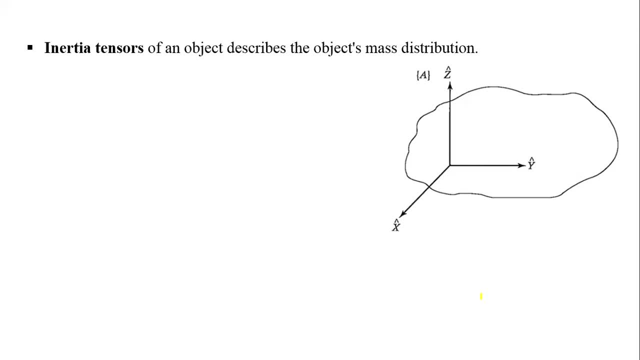 the mass matrix in manipulator dynamics theory is referred as inertia tensor. we have read the concept of tensor in our deformable bodies history. there we have learned stress tensor, strain tensor and some other tensors. in a similar fashion we will learn inertia tensor for manipulator dynamics history. 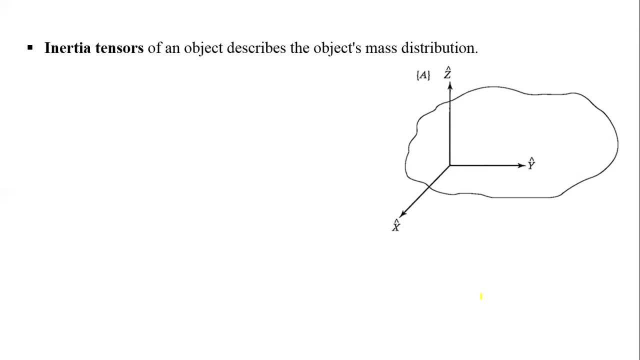 so inertia tensor is written as a 3 by 3 matrix. in this form and the diagonal elements of this matrix, Ixx, iy, y, andigence represents mass moment of energy and the remaining elements of this matrix, like Ixy, dx and Ill, accurately present product moment of inertia. sigma isurs of kanji indexes and cyclic units as the possible, both self-contained elements matter element and friendships between, and这个绯m德还是一件内部わized by this matrix, then the fundamental model oféis yy和balanced by motor shrimp engine and yy z represents product moment of inertia or of energy. 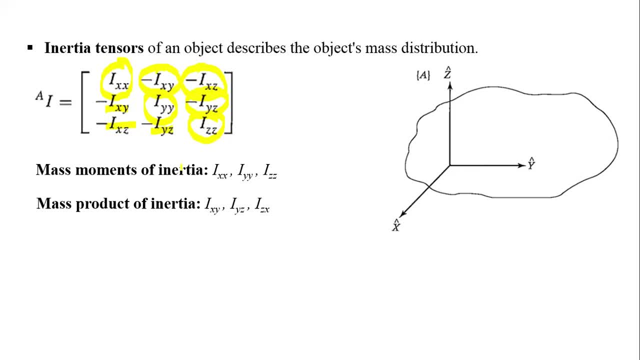 There is another very important term related to inertia tensor is principal axis and principal moments of inertia. Principal axis refers to the principal frame of reference. Before discussing this concept of principal axis and principal moments of inertia, I would like to describe this term: the inertia tensor. 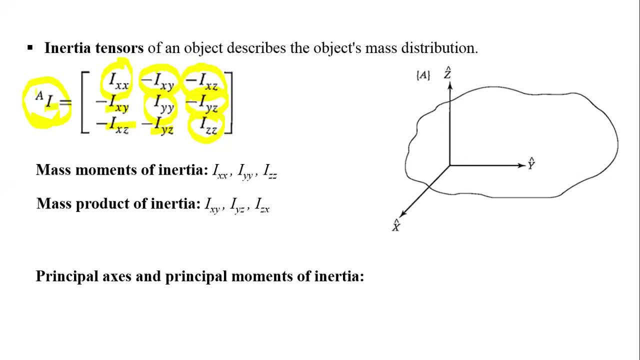 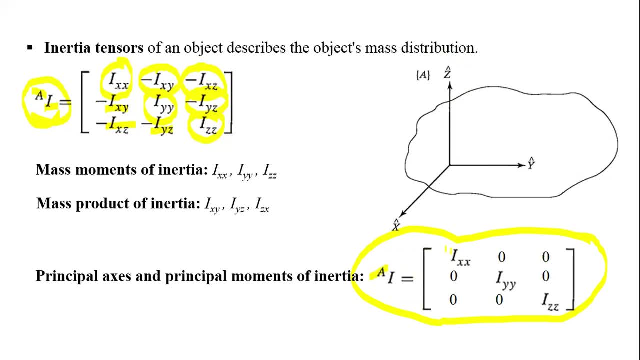 way that you get the inertia tensor as a diagonal matrix. then that reference frame is known as principal reference frame and the axis, three axis, are called principal axis. also, it is important to know that these diagonal elements, mass moments of inertia for this particular case, are called principal moments of inertia for the derivation or for the 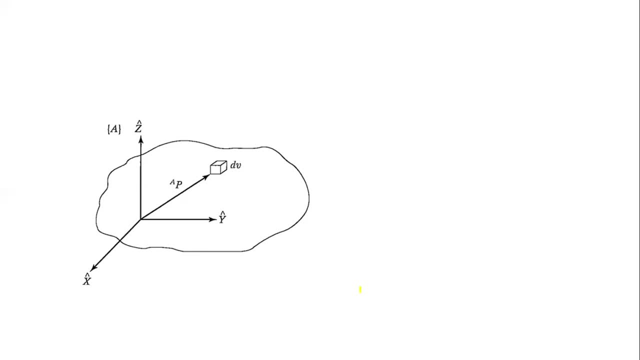 understanding of this expression. i have taken a solid of arbitrary shape and inside this solid a differential element of volume, dv. so dv is the differential volume of the element has been selected. the density of material is uniform and denoted by the variable or the constant rho, the moment of inertia about x-axis. 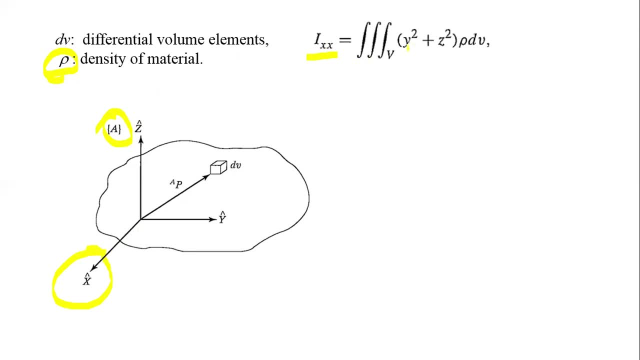 and the moment of inertia about x-axis and the moment of inertia about x-axis is calculated as the volumetric integration of the function y square plus z squared into rho. in the same fashion, the moment of inertia with respect to y-axis and z-axis are calculated. 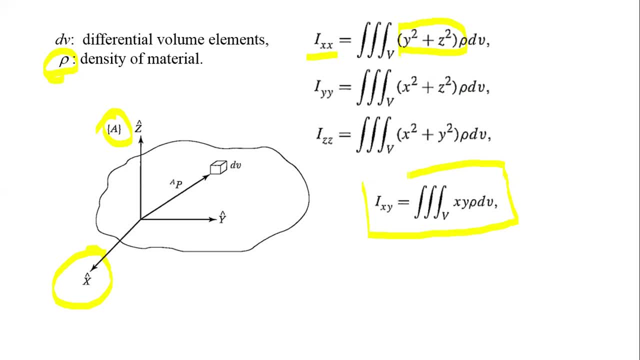 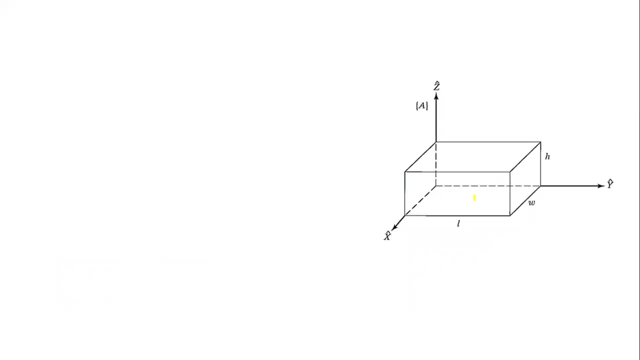 the expression of product moment of inertia is a volumetric integration of the function x, y, rho. the same way, i x z. in the similar way, i x z and i y z are written. let's use the expression of moments of inertia- product moments of inertia- written in the previous slide and apply it in this example. 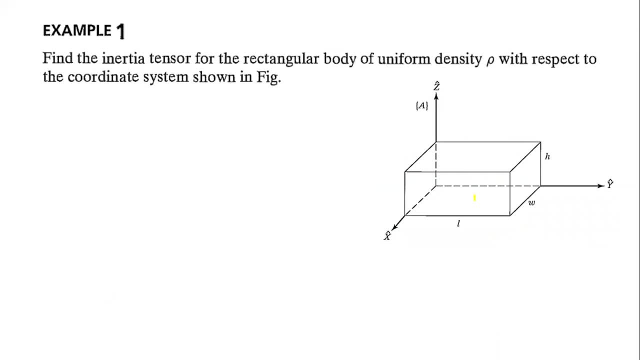 so in this example we need to find the inertia tensor and the solid is of type rectangular. for this rectangular body the density is uniform and the coordinate is equal to the coordinate system. frame of reference or coordinate system is shown here. first we will derive the moment of inertia about x-axis and the. 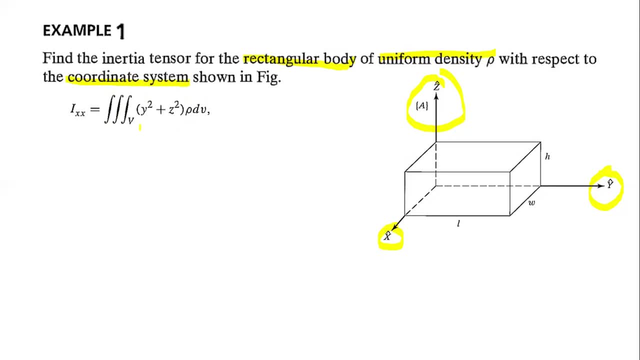 expression is like this: first of all, we need to assign the limits for each integration. before assigning the limit, let's decompose this variable, dv, into its associated components, so dv can be decomposed into dx, dy and dv can be decomposed into dv and dv, so the first integration refers integration. 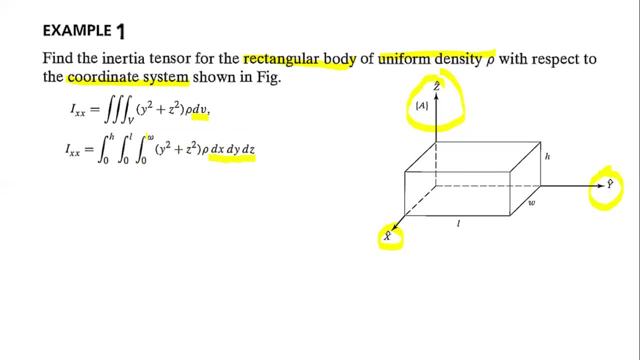 with respect to dx. so the limit will be 0 to w for this particular case. let's see in the diagram. so this x variable varies from zero to w. similarly, the integration with respect to dy takes the limit from zero to l. this is zero to l, and integration with respect to dj takes limit from zero to h. 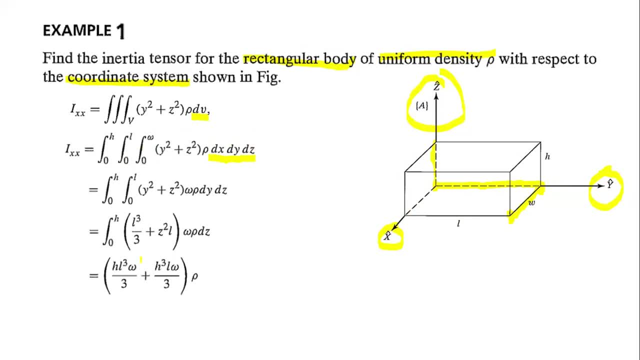 after integration we get this result: i mean i x, x is equal to m by g, l square plus h square. similarly, we can derive the expression of i, y, y and i z, j. next we need to derive the expression of product moment of inertia: i x, y, i. 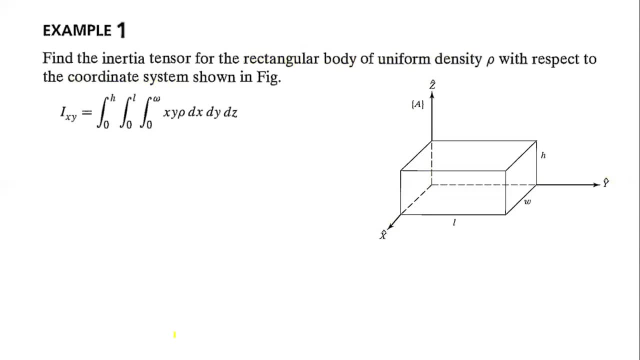 y z and i j x. here is the expression of i x y and it needs to be integrated. so after first integration we get this equation, we can integrate integration and finally, i x- y is equal to m by 4 into w- l. similarly, expression of i y z and i x z can be derived: 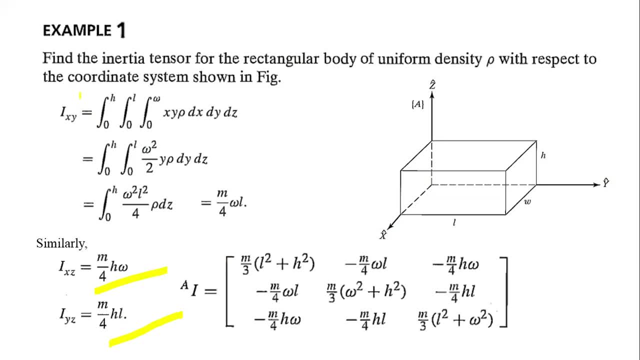 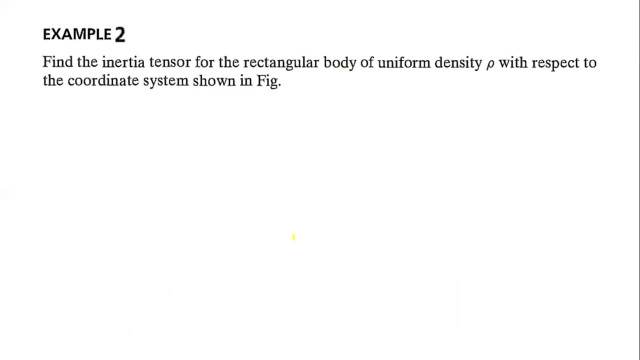 after finding the expression of three mass moment of inertia and the three product moment of inertia, we can write down the inertia tensor matrix and we will get this matrix equation. we can put mens, objects and let us this coaching from this matrix, of this particular frame of reference. 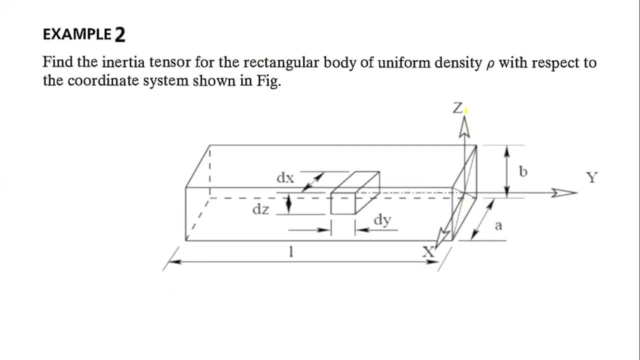 we need to find all these 것, memories and also the value of thisدes incredible space is alreadyring here, so let's find out the inertia tensor matrix for this particular frame of the body. with respect to this frame of reference, multiple space for the hair tensors of surf ad Kuja, that is, ю, and, in our model, another example. in this example, the coordinate system or khauling' r, range from here to here. we receive the thus change: 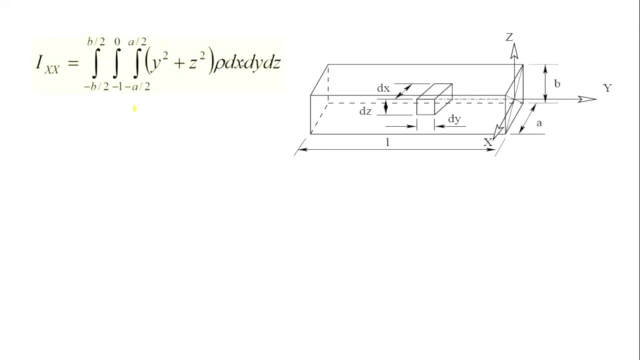 So the expression of ixx will be same as the expression we used in the previous slides. only limits will be changed. So limit for this integration with respect to dx will be from minus a by 2 to plus a by 2.. For this integration it will be from minus l to 0.. 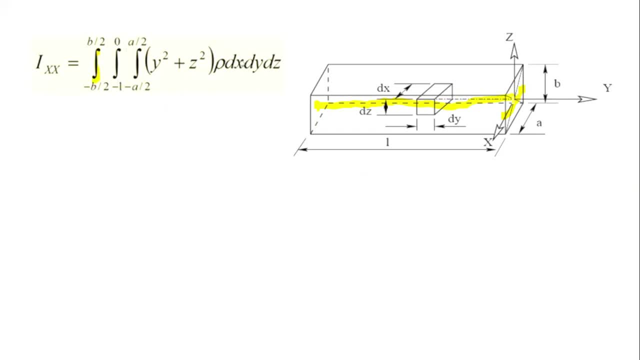 And for this integration we will get the limit from minus b by 2 to plus b by 2 along the z-axis. Finally, after integration, we get this expression as the expression of ixx. Similarly, we can derive the expression of iyy and izz. 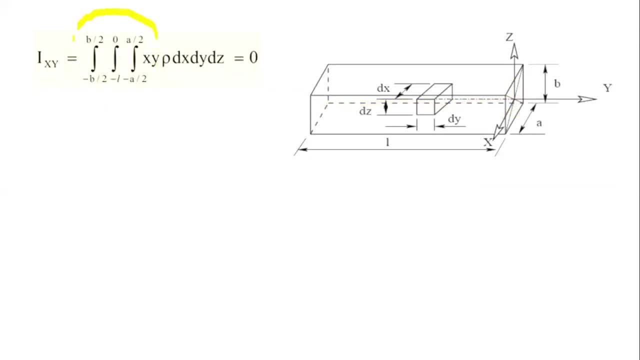 Product moment of inertia can also be generated with help of these limits And because there is a symmetry about xy-plane, we get: ixy is equal to 0.. Similarly, iyz is 0 and izz is equal to 0.. After substituting these expressions or values of mass, moment of inertia and product moment, 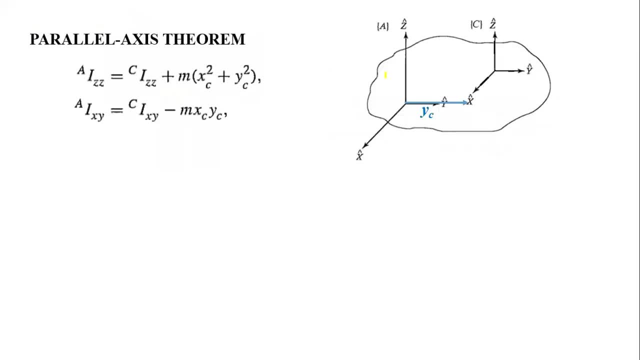 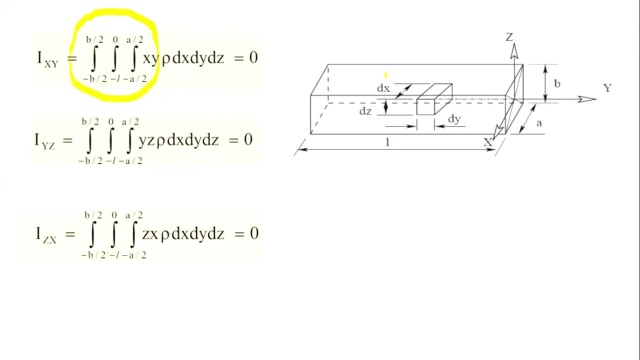 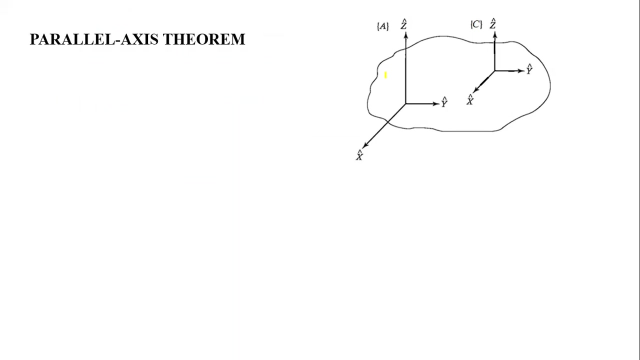 of inertia. we get this inertia tensor. Inertia tensor expression is not written here, but we can easily write all these variables to generate inertia tensor. Next is parallel axis theorem. So why this parallel axis theorem is important. In the previous slides we derived inertia tensor for two reference frames for same type. 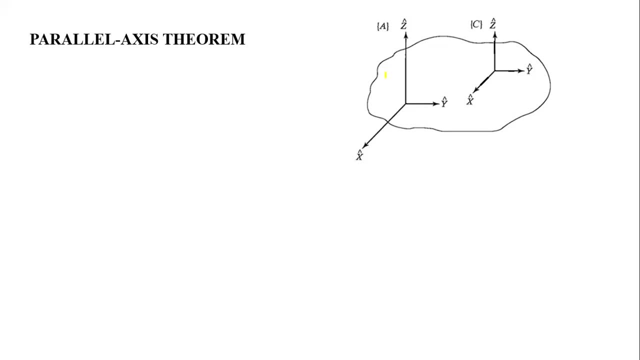 of solid. So if any solid or any object, if the reference frame is shifted, then the reference frame is shifted. So if any solid or any object is shifted, then the reference frame is shifted. So then this parallel axis theorem can be used to change the inertia tensor from one 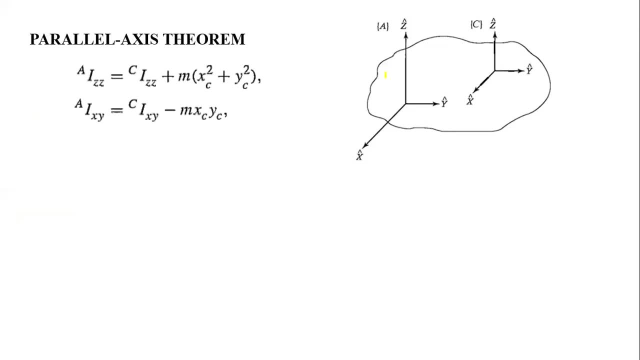 reference frame to other reference frame. So in parallel axis theorem is written like this. Let's understand this expression. So izz, basically inertia tensor about the axis z in the frame of reference A. So this is reference frame A. It is equal to the你说. 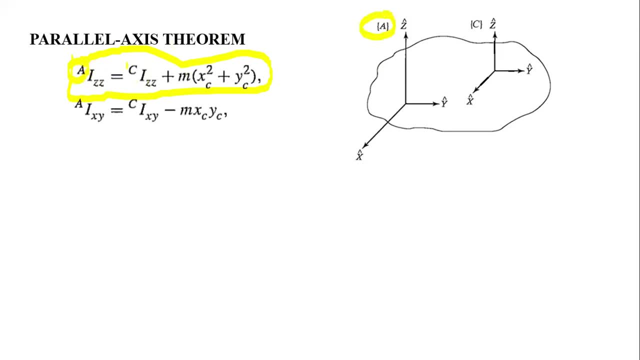 So some kind of error has been made. So what happens now? Well, the third one is d, x equals one, and then if iiot, erotica meet. So this is a normal izz with respect to frame c. so this is the new frame c. 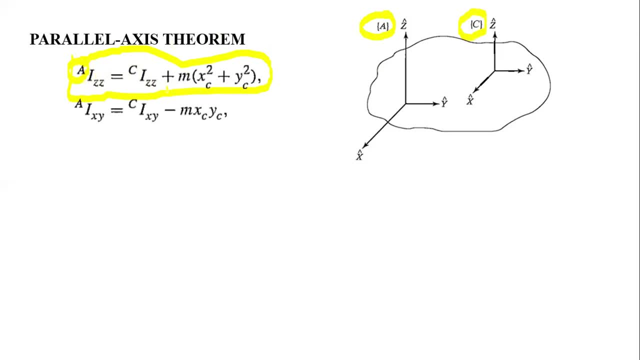 so this inner set tensor need to be added with this term for getting izz with respect to it. so what is this term? this term is very similar to m r square. m is mass of the object and this xc square plus yc square denotes this vector. so yc is this distance along the y, xc is this distance along the x. 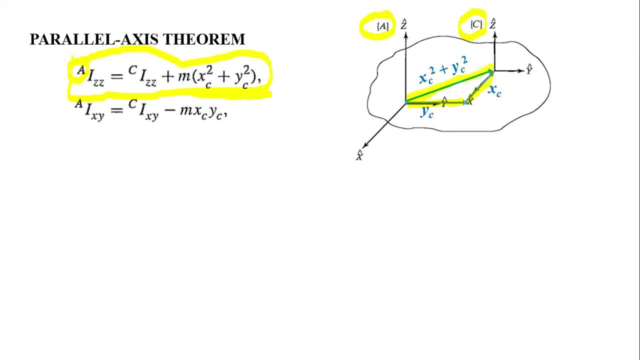 and applying pythagoras theorem, we get this position, and the parallel axis theorem for product moment of inertia is written like this: so let's take this example, and in this example the frame of reference is a, a, a and it is shifted to a new reference frame. 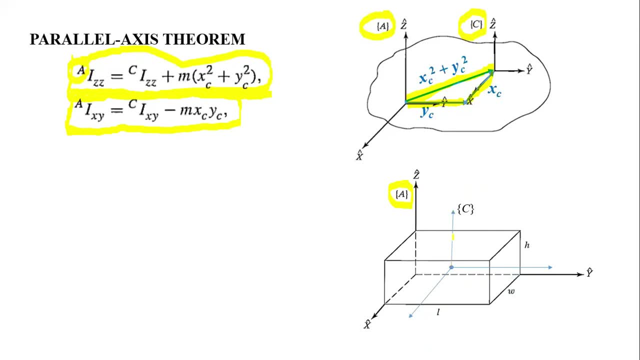 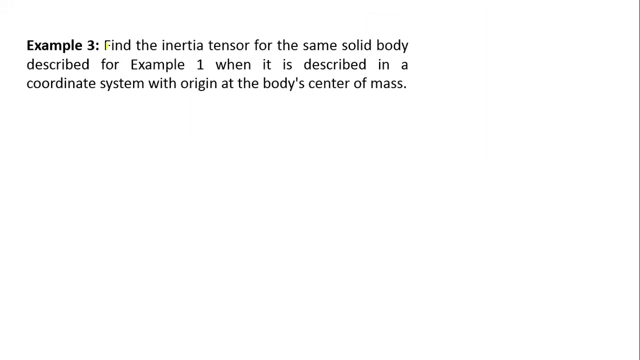 at point located at the centroid of this body. hence, the expression of all the values of xc, yc and zc will be equal to half of the w? l s respectively. let's take another example. in this example, we need to find the inertia tensor for a rectangle. 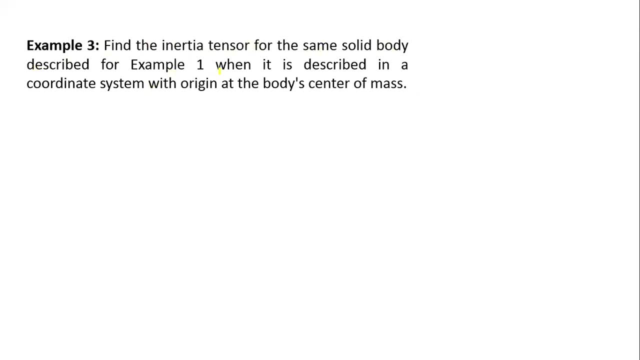 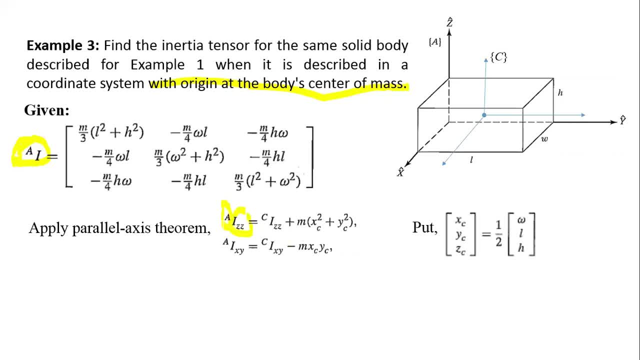 a is known and if we subtract this izz with respect to a, if we subtract m, xc square plus yc square from this term- izz with respect to a- then we will get izz with respect to c, xc. yc can be obtained from this expression and the resulting intercept answer with respect. 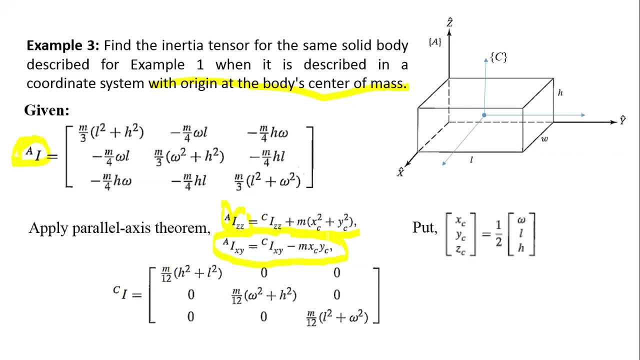 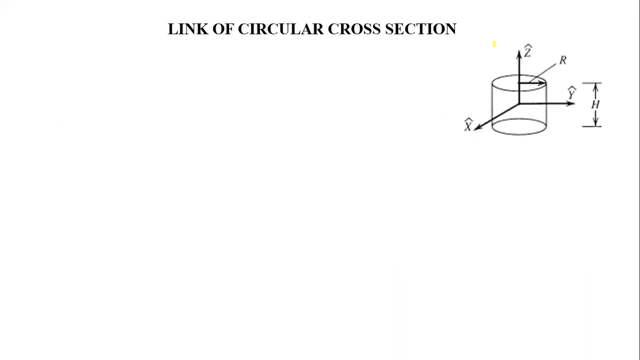 to c frame will take this form: this is the expression of parallel axis theorem bar called product. moment of mercedes means: after this substitution or after this shifting of frame of reference, we got principal reference frame. so this c reference frame denotes principal reference frame. let's take another type of link, and this link is of circular cross section. 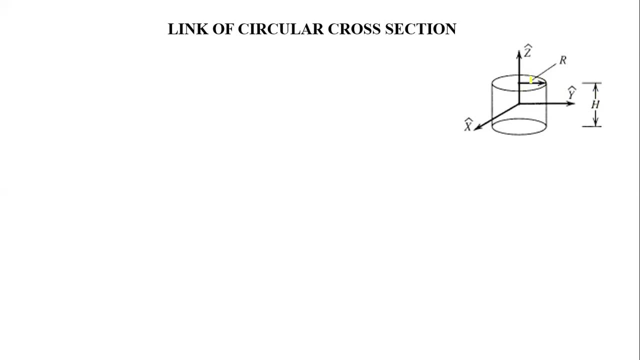 the height is h and the radius of this cylindrical or circular cross section is r, we need to find the inner set tensor for this body with respect to a frame with origin at the center of model. so here we got the expression of i zz. so in the previous expression, the function which 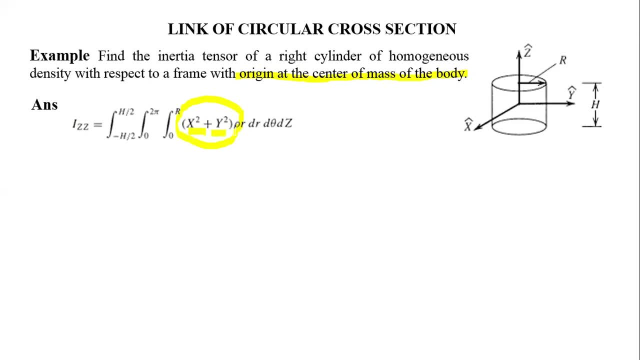 needs to be integrated was x square plus y square into rho. so this is the expression of i zz. so in the previous expression the function which needs to be integrated was x square plus y square into rho. so this x square plus x square into rho equals r and integration. 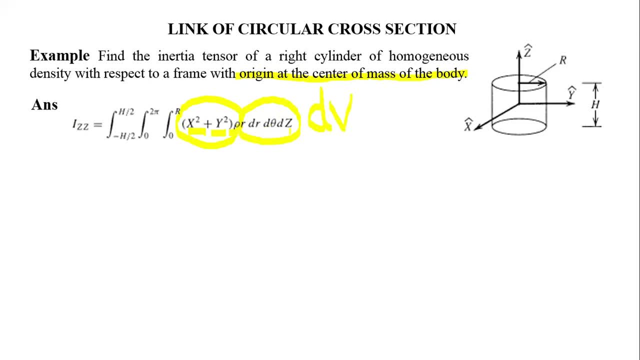 was done with respect to dv. so here basically dv is written as r into dr, into d theta, into dz. so this r, dr, d theta is basically denoting area of the differential element and if you multiply area with dz you get differential value. so if you take any differential frame, 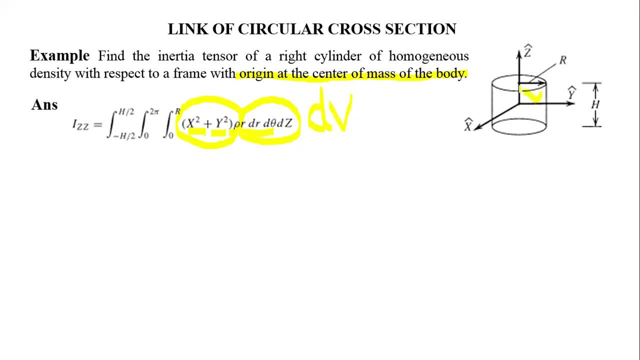 element along the circumference and if it imposes a angle d theta, then rd theta is basically arc and this arc length into dr. dr represents area of this differential element and the digit dz along the height of this cylinder. this is the height, the length along the height of cylinder. 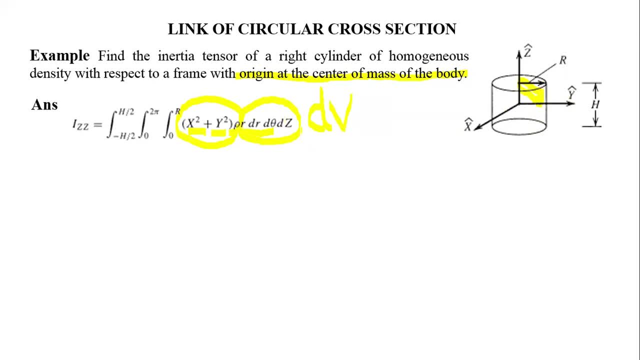 so if you multiply this area by digit, you get the pencil value. next we need to assign the limits for each integration. so limit for this integration will be from 0 to r because it is with an integration with respect to dr, so dr varies from 0 to r. this integration is done with respect to d, theta and 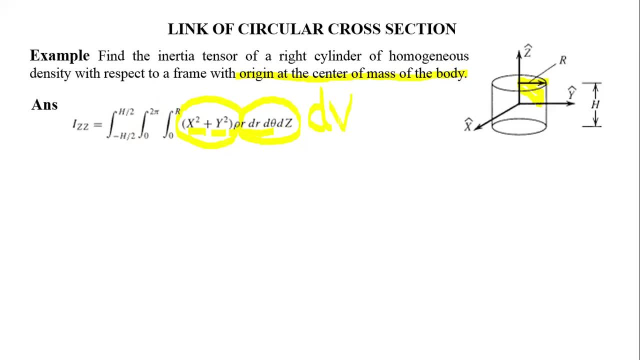 d theta varies from 0 to 2. pi dz varies from minus h by 2 to plus h by 2. so integrate it and substitute: x is equal to r cos theta. y is equal to r sine theta. how we got this expression? so suppose you are taking this differential element at an angle- theta with respect to x axis from here. 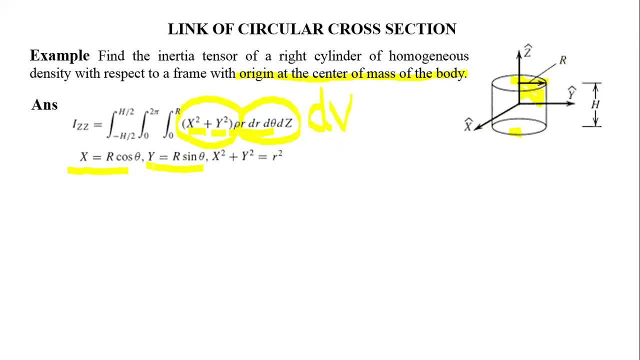 so the x component will be r or theta, and y component will be r sine, and x square plus y square is equal, will be equal to r square. substitute these expressions in this integration equation and we will take this as the resulting expression, and we will take this as the resulting. 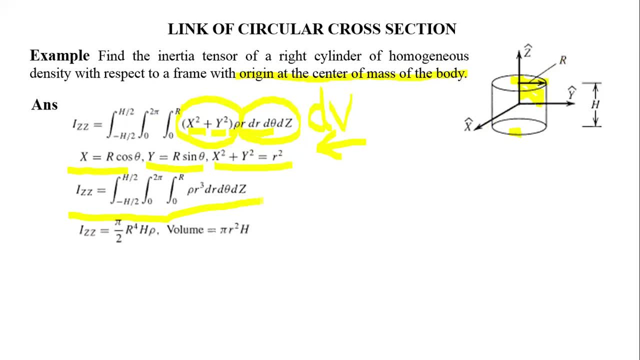 expression of mass moment of acceleration. after integration we get this equation where volume is pi r square h, and if we substitute, then i z z will be equal to half m r square. this r square can be written as capital r square. similarly, we can find out the expression of i xx. 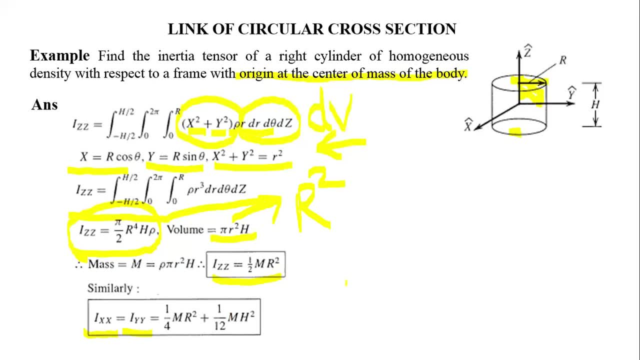 and i- yy. they will be same because of symmetry. from symmetry we can find out that the product moment of inertia, for this particular case, will be equal to 0. so i x- y is equal to i x, z is equal to i y, z is equal to 0. 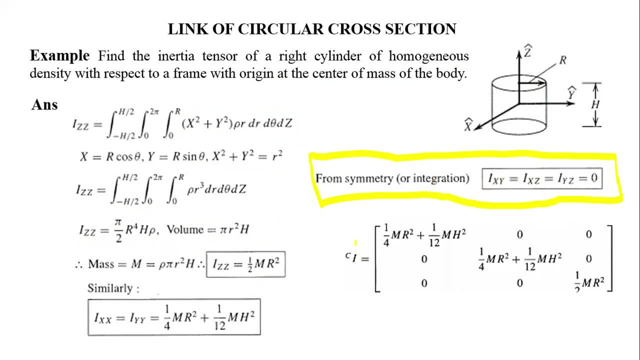 substitute these values or equations of moment of inertia and we will get inertia with respect to c. in case of slender link, the value of h or height of the link is very large as compared to the radius, so we can ignore this term from the inertia tensor and the resulting inertia tensor will be. 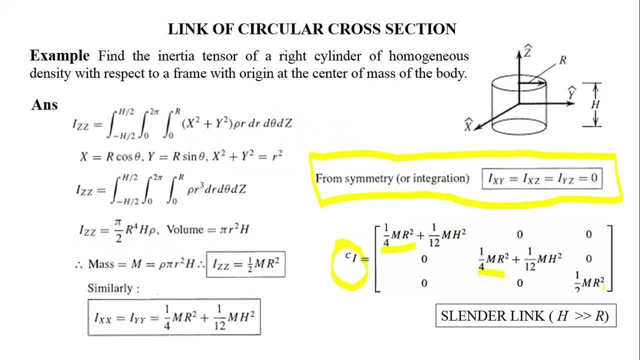 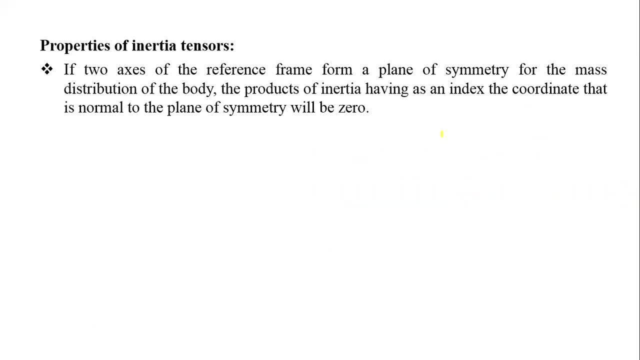 1 by 12 m h square, 1 by 12 m h square, 1 by 12 m r square in the diagonal, and the remaining element will be gd. we searched for gd, so anyways, h is a PA that consists of a number of velocities, times, k. 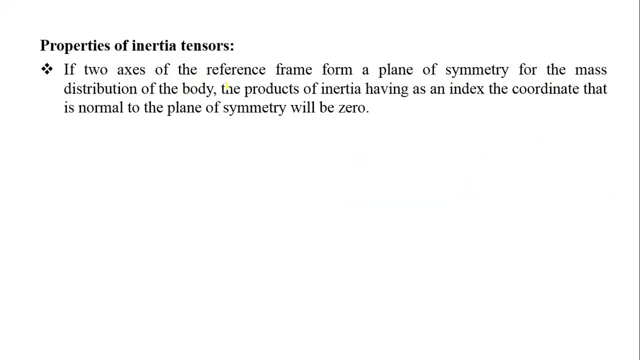 where k? perhaps we have k as a säga, but if we divide k by 2 and mS as ainator, we should have 1 on both sides. so now we know that if we take themax variable at any of these points, we get cen in consequence of: d is equal to m. 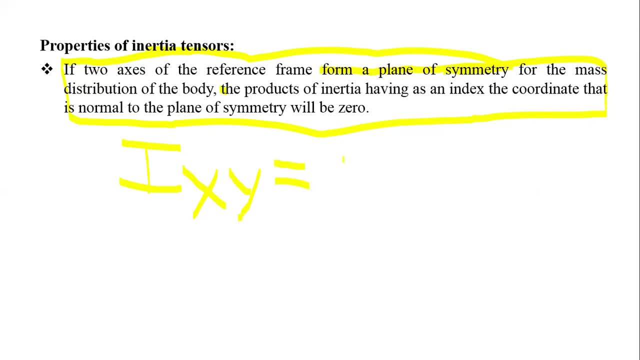 then we gave product motion for principle of dy. So here now, if y is px and y is plane of symmetry of inertia is equal to zero. product of inertia is equal to zero. another property: moments of inertia must always, be, always be positive, but product of inertia may have either sign.